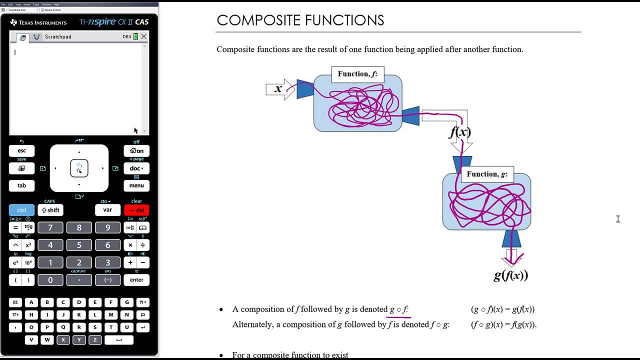 Now I must say VCAR don't tend to use this notation in the exam, but it is really common in your textbook And it is coming in in the study design change. So GOF is g of f of x. that's how I would read that. 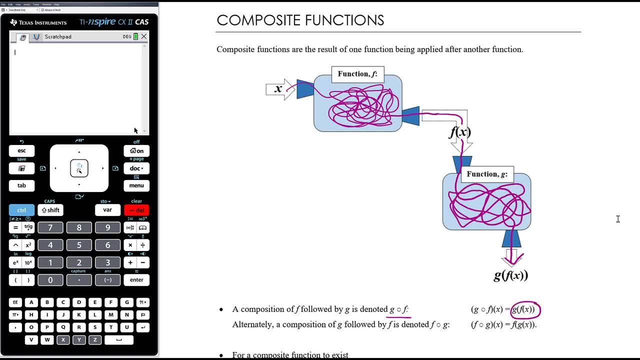 And so we would write that like this: g of f of x, okay, Substituting f of x into g of x. We're subbing x into f to get f of x and then subbing f of x into g to get g of f of x, okay. 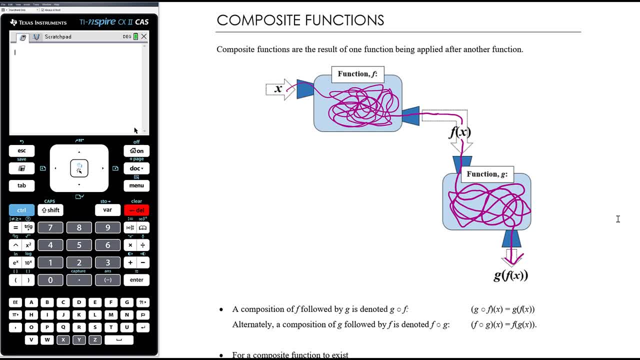 If we compose the functions in the reverse order, a composition of g followed by f is denoted by FOG f of g of x, and that's where we take x. we sub it into g first, this time to get g of x. 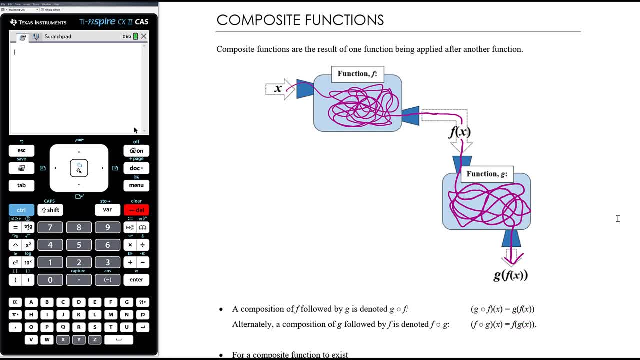 and then we sub all of that into f to get f of g of x, f of g of x, FOG. So that is when g is being applied first and then f. Okay, there's a really important moment that happens here, okay. 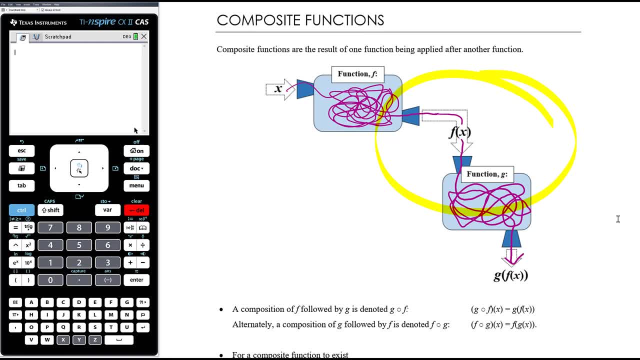 that we need to ensure works correctly in order for the composition to exist. So what we need to understand is these x values here that we start with they, we call the domain of f, and it gets subbed into f. f turns them into new numbers, which we call the range of f. okay, 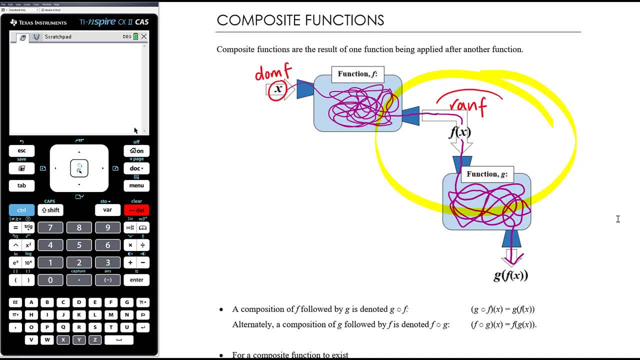 But then we're going to make the range of f become the domain of g, So the range of f has to be able to be the domain of g, And so what that means is that the composition can only occur is if the range of g is the domain of g. 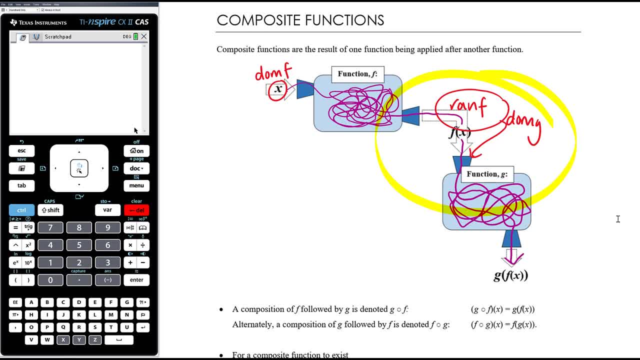 So the range of f is a subset of or equal to the domain of g. okay, If, for example, the domain of g is only r plus and the range of f is r, we're going to have a problem because we've got numbers coming out of f. 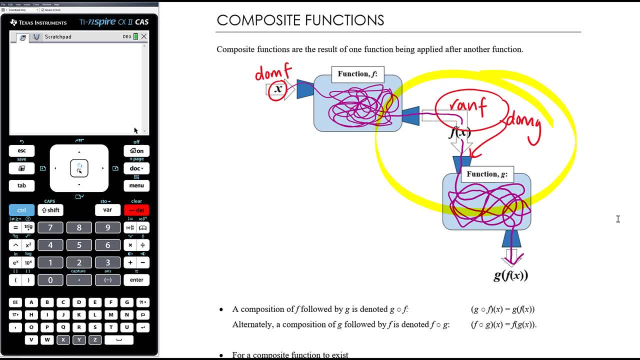 that cannot be substituted into g, okay, So it's all about ensuring that that issue in the middle there can be dealt with. So the range of the first function, or when we look at it in this notation, it's going to be g of f of x, okay? 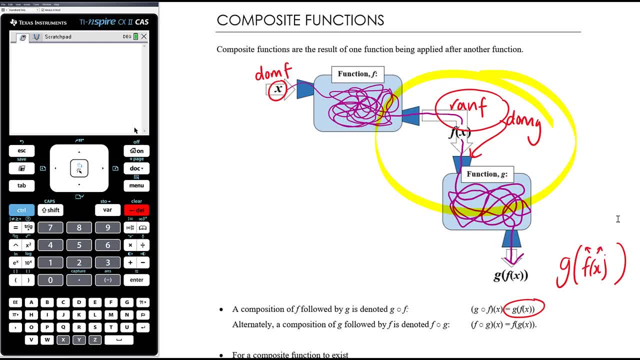 The range of the inside function. so all the numbers that are going to spit out of f, they have to be able to fit into g, So they have to be a subset or equal to the domain of g. okay, So for a composition to exist. 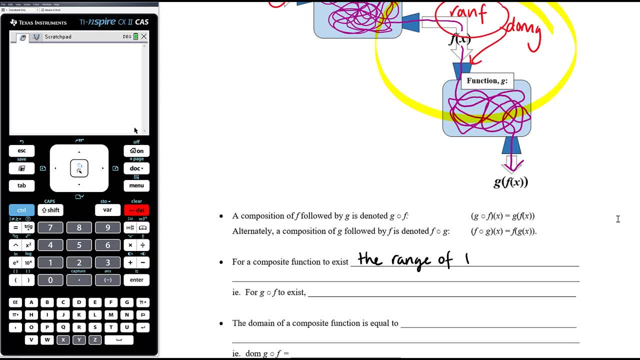 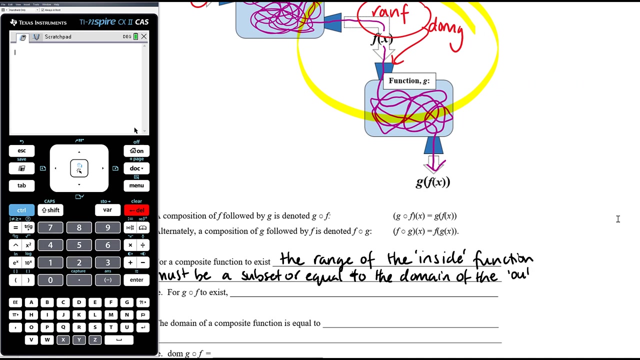 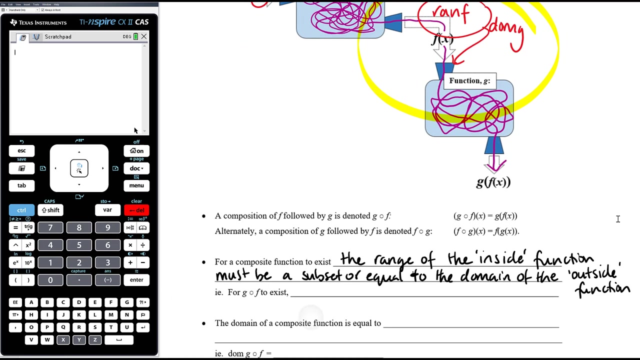 the range of the inside function- I'll use that term inside loosely- of the inside function must be a subset or equal to the domain of the outside function. okay, So if that doesn't happen, then we cannot perform the composition, We cannot calculate GOF or FOG, depending on what it is. 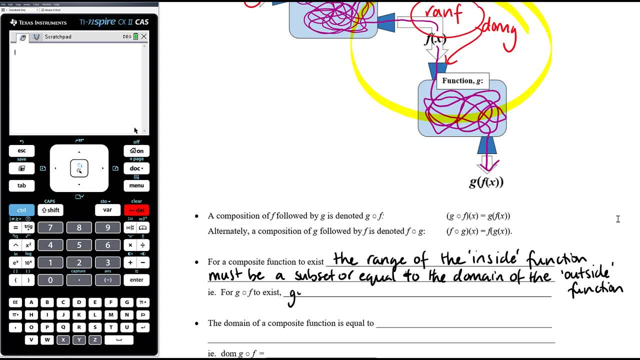 So for GOF to exist- remember GOF of x is g of f of x, So f of x is the inside function- We need the range of f to be a subset or equal to the domain of g, And if it's not, then the composition can't occur. 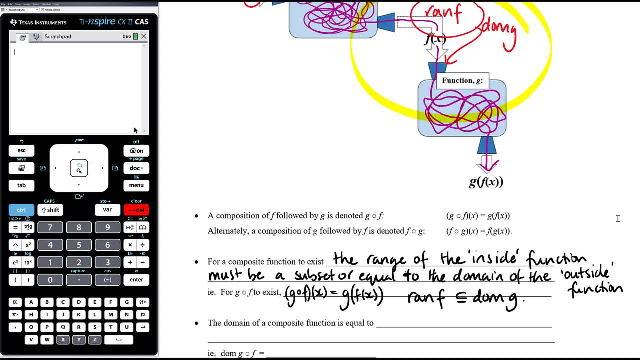 Or we need to restrict the original domain of f so that the range of f isn't so large, so that it instead will become a subset or equal to the domain of g, The domain of a composite function. so let's go back to our machine up here. 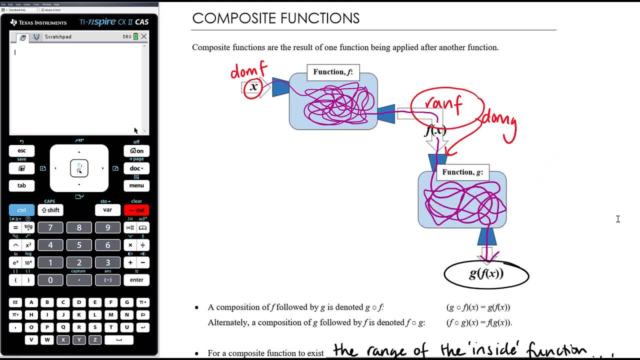 So the domain of GOF g, of f, of x: here's the x values we started with up here. The domain of the inside function, that's the original x values that get subbed in right at the beginning. that is the domain of the composite function. okay, 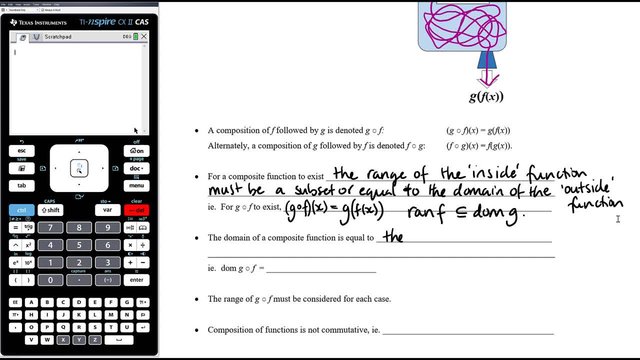 So the domain of a composite function is equal to the domain of the inside function. So domain of GOF, remembering that GOF is g of f of x, so f is the inside function. So the domain of GOF is just equal to the domain of f. 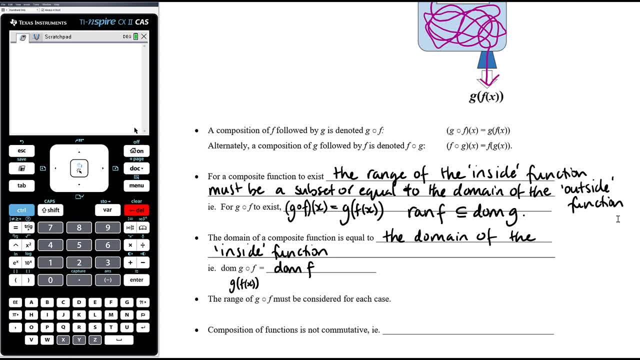 The range of GOF must be considered for each case. So you must then think about: okay, well, what domain did I start with? and given the rule that I've ended up with for GOF, what does that mean for the range? So you've got domain and rule. 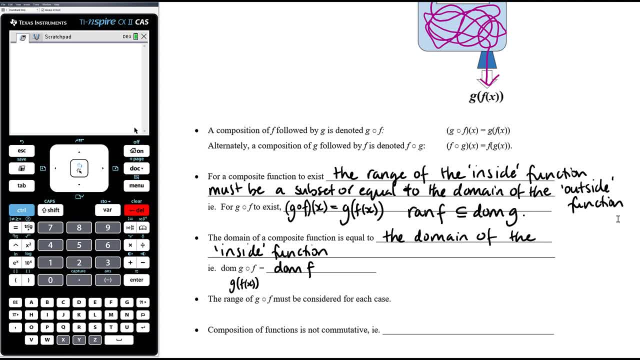 those things together must be combined for you to be able to think through what the range is going to look like. Composition of functions is not commutative. Okay, so let's talk about that word: commutative. Addition is commutative. multiplication is commutative. 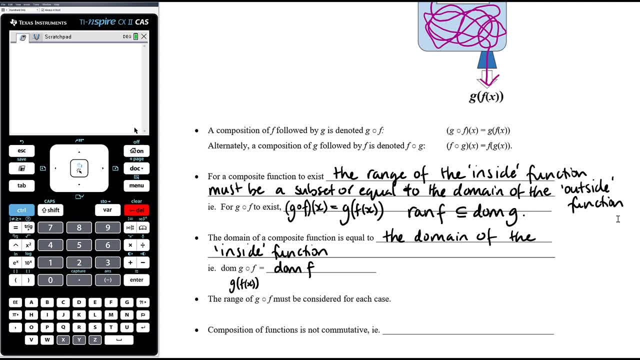 subtraction is not commutative, division is not commutative, So it's about whether you can reverse the things. So, for example, 2 plus 3, 3 plus 2, they're the same thing. it's a commutative operation. 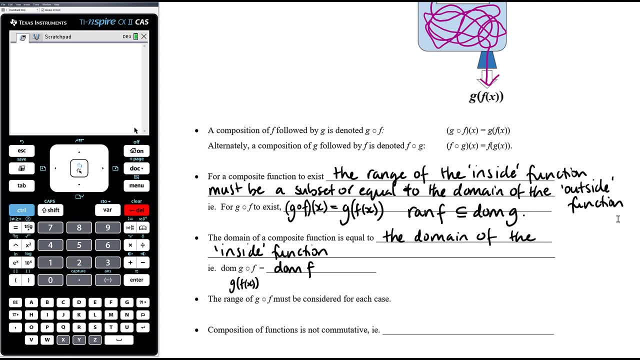 2 times 3,, 3 times 2, they're the same thing. it's a commutative operation. However, 3 minus 2 and 2 minus 3 does not give the same thing. Subtraction is not commutative. 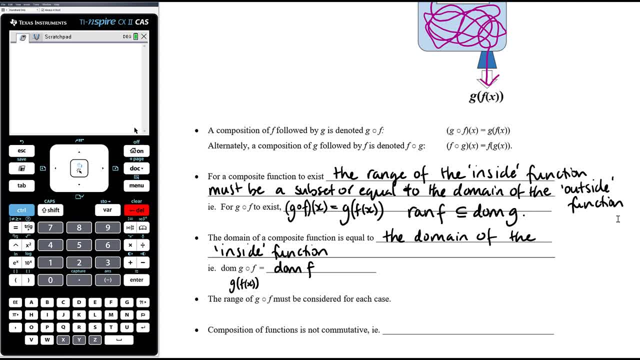 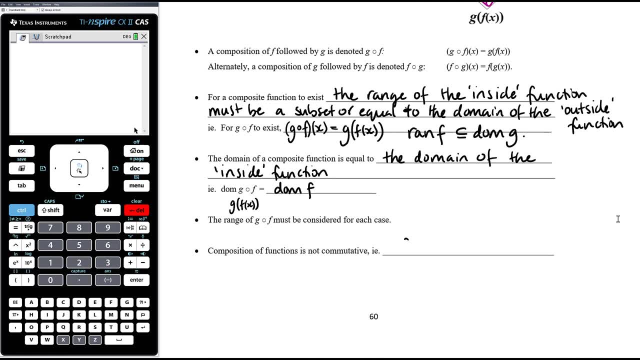 Again. you know, 2 divided by 3 is not the same as 3 divided by 2. Division is not commutative, So composition of functions is not commutative. That means that fog of x is not the same as goth of x. 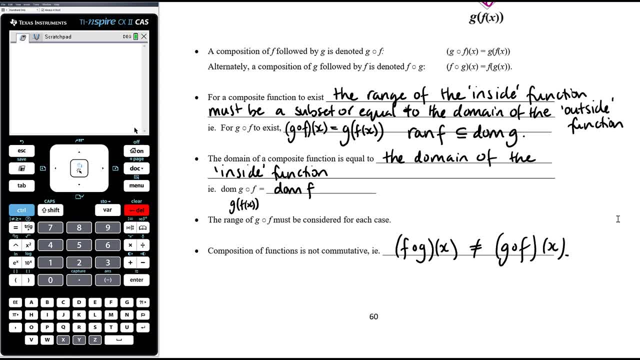 And in some cases, one of those things might be possible: Fog might be possible, but goth might not be possible, or vice versa. And certainly, even if they're both possible, we would get different rules. Okay, let's work through some examples here. 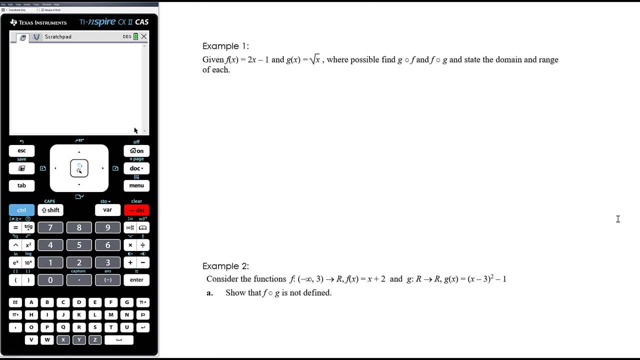 So, given that f of x is a simple linear function- 2x minus 1, and g of x is a basic square root function, where possible find goth and fog and state the domain and range. Okay, so it's really important before you launch into any algebra. 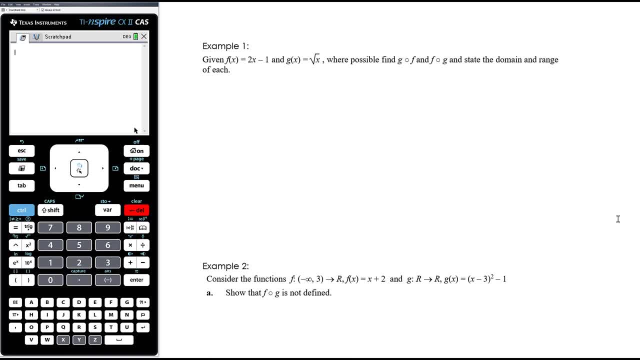 to consider whether or not the composition can exist at all. So let's think those things through, and we're going to need to be able to think about domains and ranges. So I'm going to just articulate: Well, let's think about goth first. 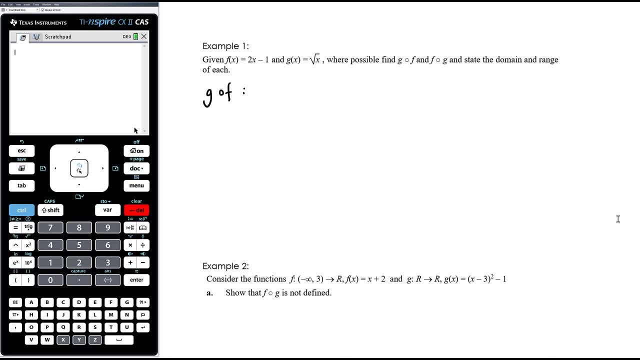 Okay, So for goth, f is the inside function. It's g of f of x. Okay, So it's g of f of x. So f is the inside. We're going to need the range of the inside function to be a subset of the domain of the outside function. 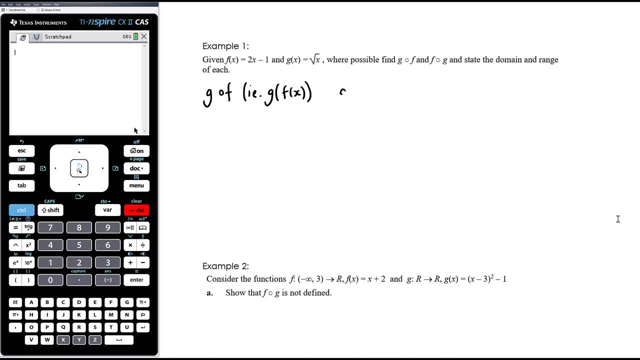 Okay, So let's consider what those sets are first of all. So sorry, we don't need domain of f, We want the range of f. So f is a linear function. So the range of f is r And the domain of g. 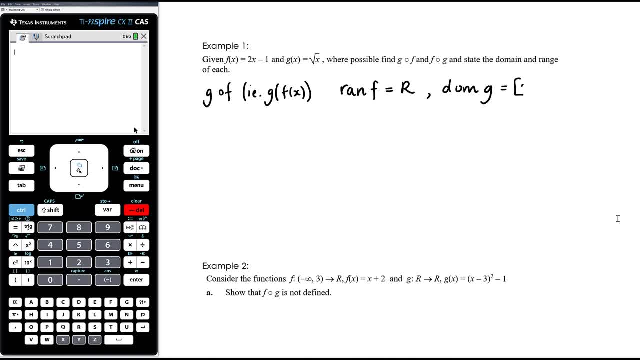 Now, g is a square root function, so that's 0 to infinity, inclusive of 0.. Okay And so, since the range of f is not a subset of the domain of g, goth is not defined, So we're not even going to try to calculate it. 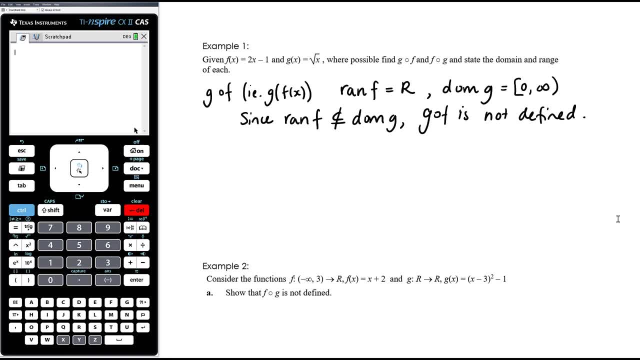 We're not going to work it out. We can't state its domain and range. It's not defined at all. Okay, So that was goth. Let's now think about fog. Okay, So fog is f of g, So we want the range of the inside function. 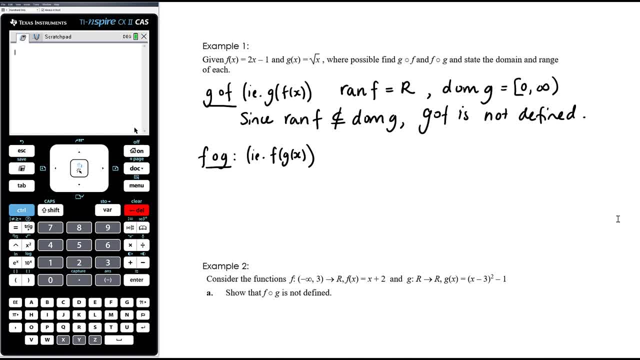 the values that spit out. So we put x into g, g spits out its range, And then those numbers need to be able to go into f, And so we need the range of g to be a subset of the domain of f. 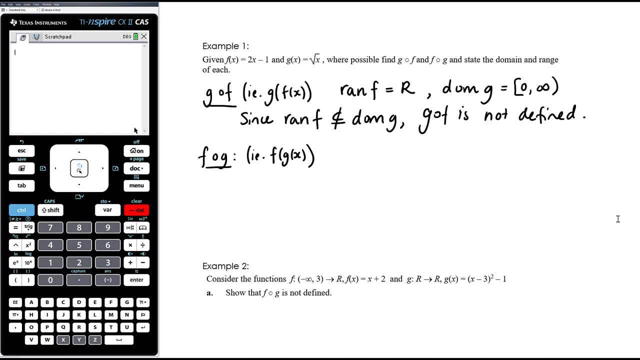 So we need to calculate those things. So range of g in this case. Now, g is a square root function, Remember, it looks like that. So its range is from 0 to infinity And the domain of f, That's a. 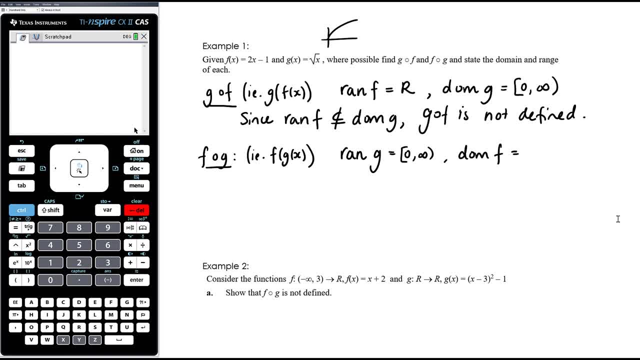 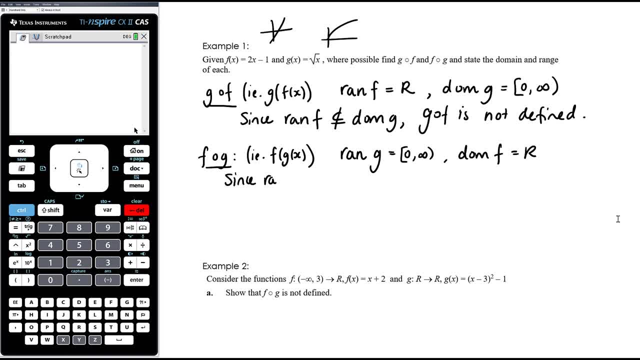 Okay. So since the range of g is a subset of the domain of f, fog is defined. It's really important if you're going to justify whether or not fog or goth is defined, you can't just say that the range is. 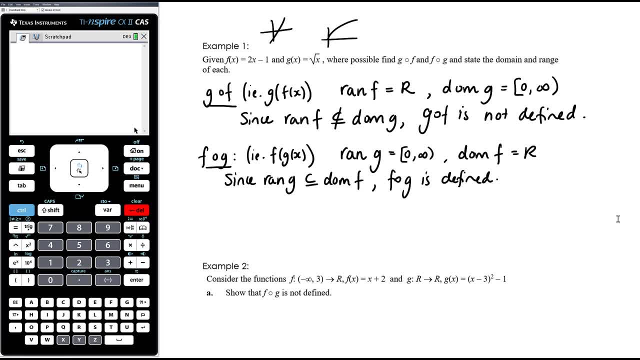 The range of this is or isn't a subset of the domain of this, without actually stating what those ranges and domains are? Okay, You must make your answer specific to the question. It's not just about making a generic statement about composite functions. You must actually think about the functions involved here and calculate the relevant domain. 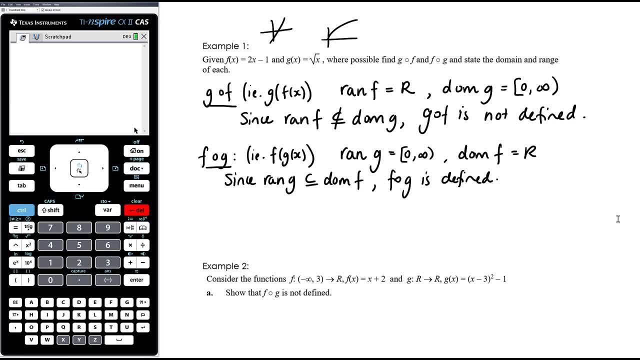 and range for those functions and draw a conclusion from that about what that means as to whether the composition is possible. Okay, So this one is defined, So now we're going to calculate it. Okay, So f of g of x means f of g of x. 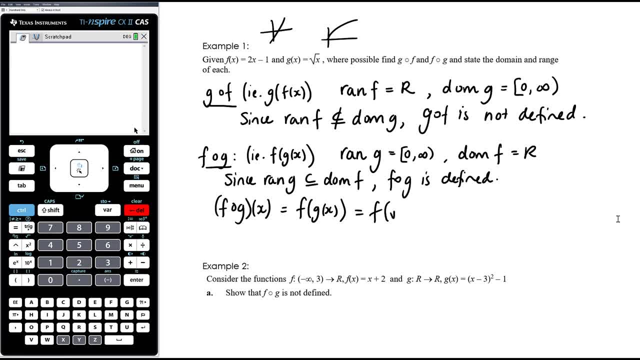 Okay, Which means f of square root of x, which is g of x, And f of x is 2x minus 1.. So our rule here is going to be 2 times the square root of x minus 1.. Okay. 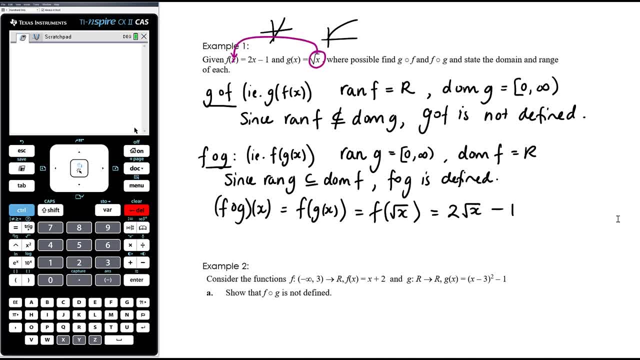 So what we're doing is we're substituting g into f. So everywhere there's an x, we're replacing it with a root x. Okay, If it was the other way around, if the composition of g, of f, of x had worked, we'd be taking 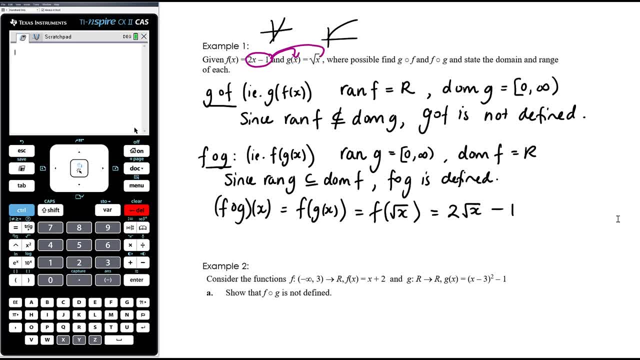 f and subbing it in place of x. So it would be square root of all of 2x minus 1.. Okay, So again you need your function. notation needs to be good to understand what's happening here. So we've calculated the rule. 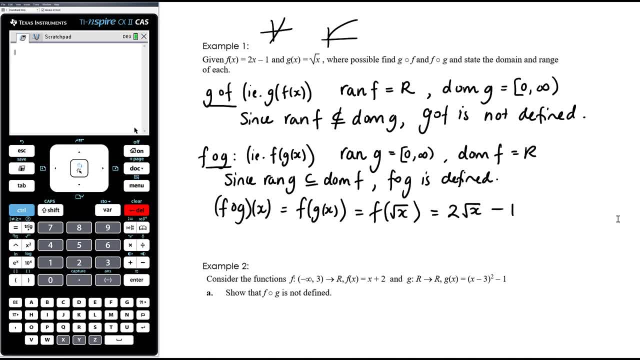 So we've found fog, which is 2 root x minus 1.. The domain of fog is equal to the domain of the inside function, which in this case is g. Okay, And g is our square root function, So it's domain goes from 0 to infinity. 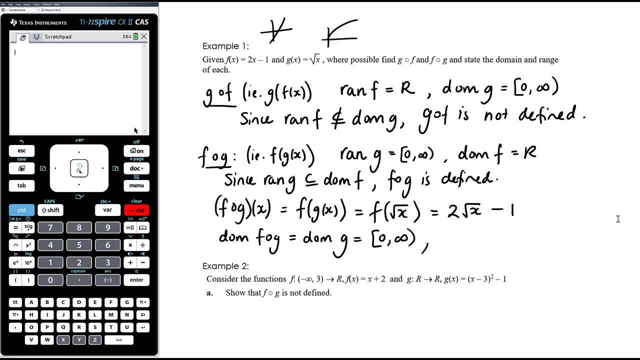 Okay, And then we want to think about this domain coupled with this rule, in terms of what that means. So, thinking about this, this is 2 times the square root of x minus 1.. So it's the square root graph dilated by 2 from the x-axis and translated down by 1.. 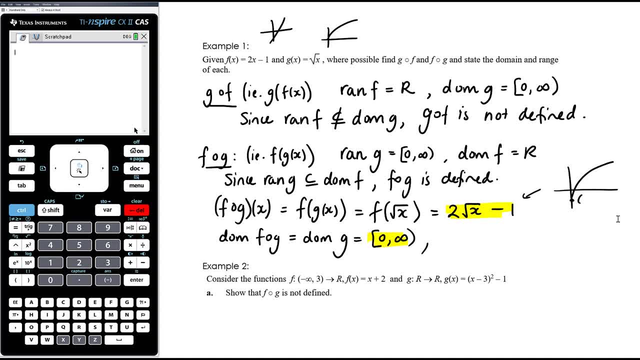 So it's going to look something like that: That's 0, negative 1.. Okay, a negative one. so the domain of g isn't in any way a restriction of that. that's, in fact, the implied domain of that rule, and so the range of that is going to be, so range of fog is going to be from. 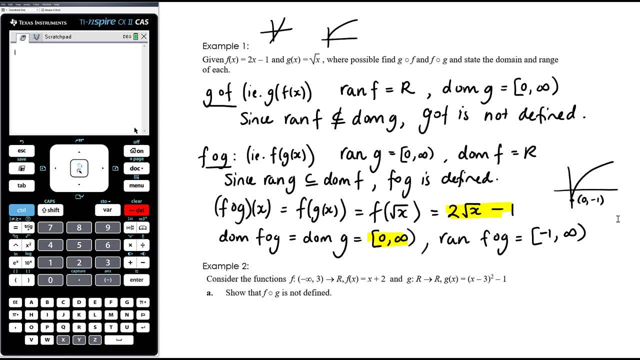 negative, 1 to infinity. best way to think about ranges is: you really do need to be able to picture the graph on what's going on. okay, so, in terms of answering our question, we've got the rule for fog- sorry, where possible, find fog. so we've determined that fog is possible. 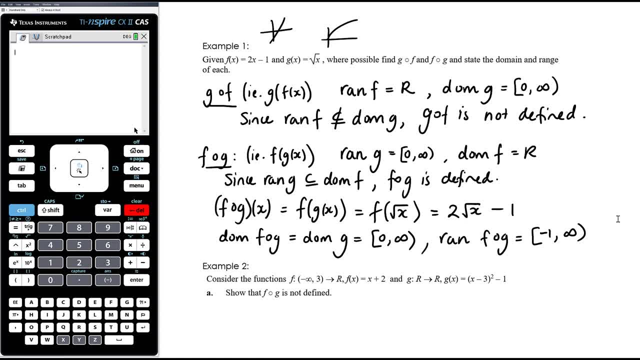 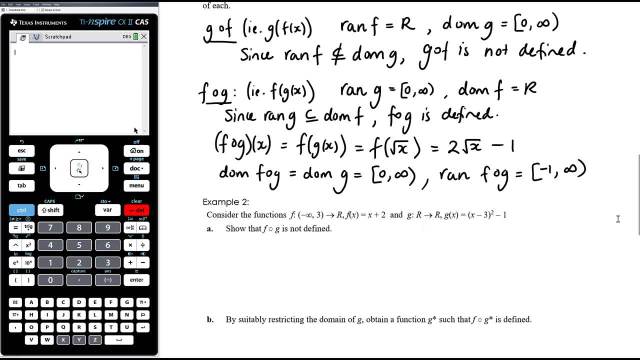 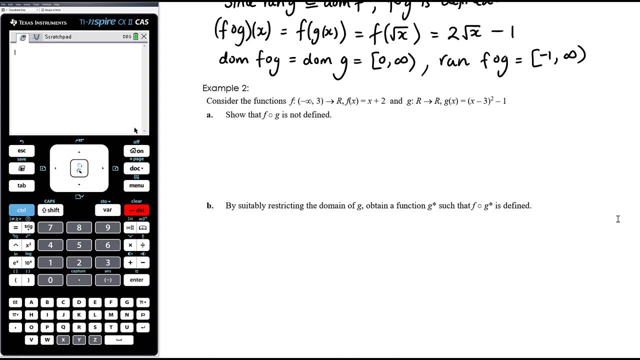 we found fog state the domain and range. okay, gof, we've determined, is not defined and so there's no need to determine its rule and state its domain range. okay. example two: consider the functions f of x equals x plus two, but over a restricted domain from negative infinity to three. 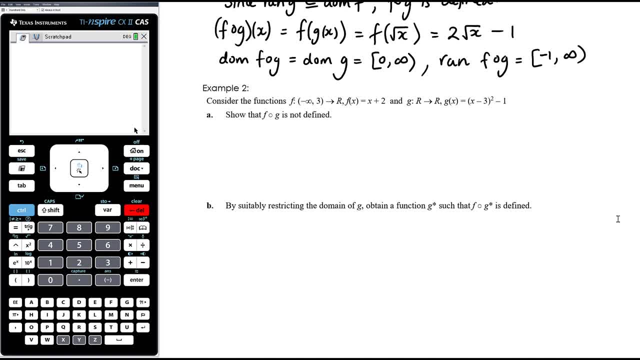 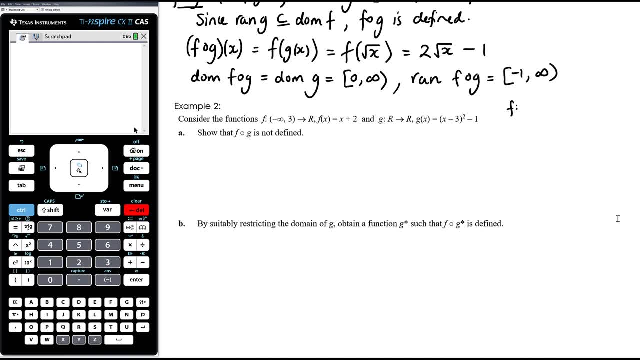 and g of x equals a parabola in turning point form. so x minus three, or squared minus one. okay, so let's just think about what these look like. so f is a straight line graph. y equals x plus two, but we're only looking at that. 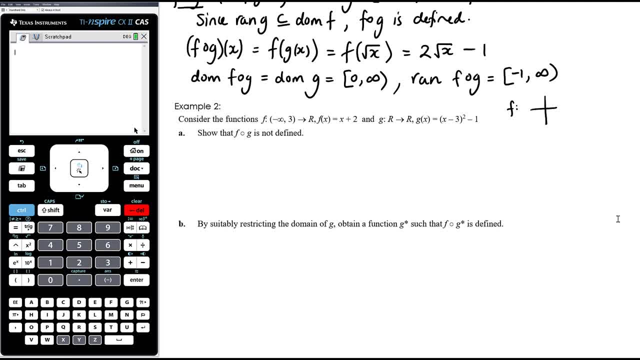 from three negative infinity up to three. so it's going to stop at three, not including three. so we're gonna have a hollow circle there. um, when x equals three, y will be five. okay, so it's going to essentially have a domain from negative infinity to three and a range from negative infinity to 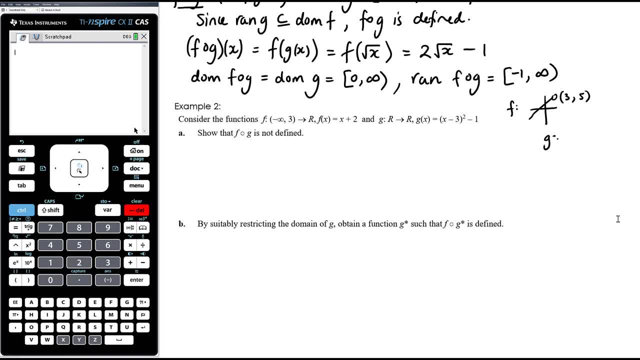 infinity to five. g is a parabola, right by three and down by one um, so it's going to be three one, three, negative one. sorry, so no domain restriction. domain is r, um, but range, because it's a quadratic, a parabola, is from negative one to infinity. okay, so show that fog is not defined. okay, so this is. 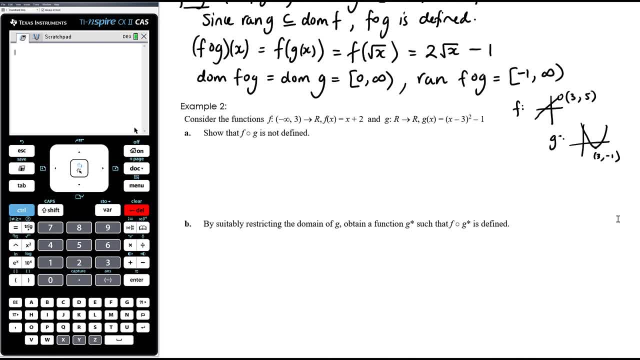 what i was talking about before. it's not enough just to state a generic statement and say that fog is not going to find because the range of g is not going to be defined. it's not going to be defined a subset of the domain of f. you have to actually state what those relevant sets are so that it's 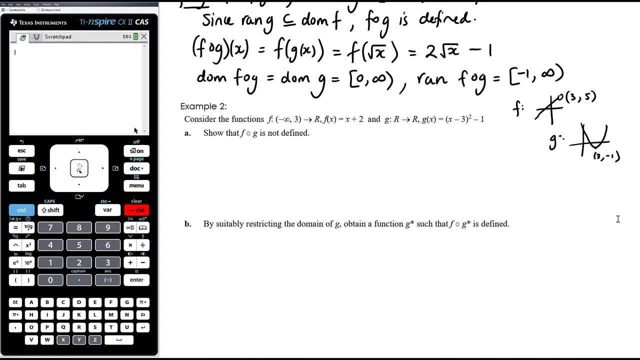 you've actually applied it to this problem. okay, so f of g of x is f of g of x. okay, so we're interested in the range of g in the domain of f. so the range of g we know is from negative one to infinity, looking at our graph and the domain of f. so i'm just going to move that out of my way. 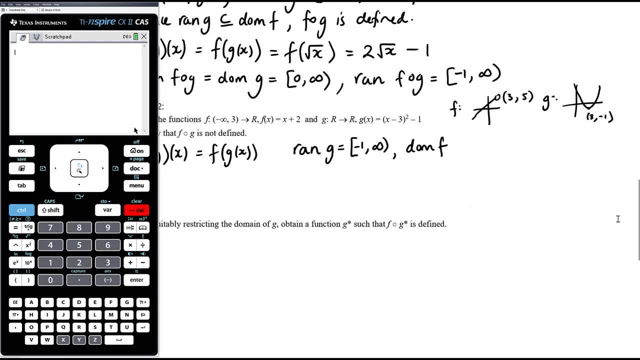 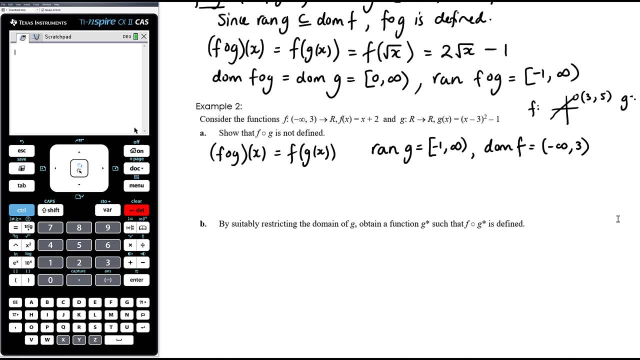 domain of f is also restricted because of the- uh we're actually given the restricted domain, sorry. domain of f is from negative infinity up to three, not including three. okay, so negative one to infinity is not a subset of negative infinity to three. there are numbers in this. 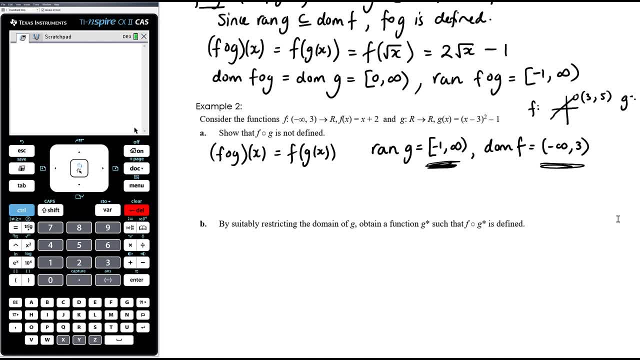 set that don't fit into this set. for example, positive five fits in here, doesn't fit in here, okay, so therefore, this does not fit entirely into here and so therefore it's not a subset. okay, so therefore, since the range of g is not a subset of the domain of f, fog is not defined. but, as i said, 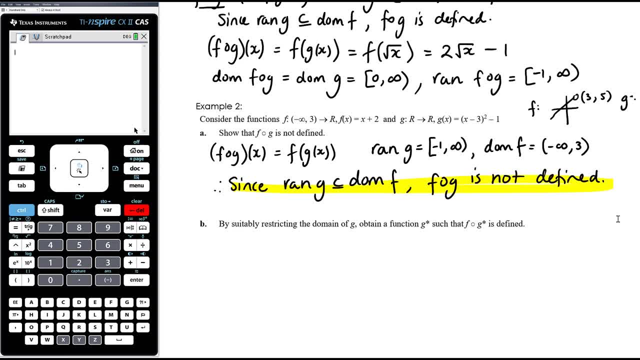 you can't just make this statement without actually providing these sets. okay for this specific example. all right, um, okay. so then part b. this is quite a common kind of question. restricting the domain of g, obtain a new function, g star. so just a modified version of g with a. 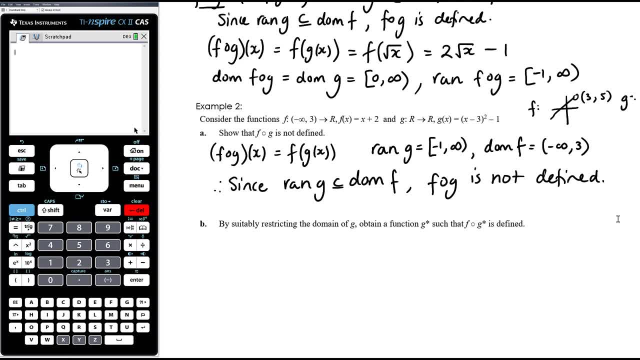 restricted domain such that f of g star is defined. okay, so f of g is not defined because the range of g is too big to fit into the domain of f. okay, so now i'm going to also say: i often say things to make this more understandable to you, but it's not acceptable to write down, you know. the domain of g doesn't fit into. we want to talk mathematically. you don't talk about it being a subseincome, so let's talk about only terms and particularVEF. as we will fit into. we want to talk mathematically. we'll talk about it being a subseotalanging rate, potentially. it's. we want to talk mathematically, we want to talk about it being a subset of these things of g and questions like that. we want to talk about two pillars, which 16,288 fazla, and how do they've involved snack permett? restart the domain of g, because our initially have defined less IdentändeltronF. 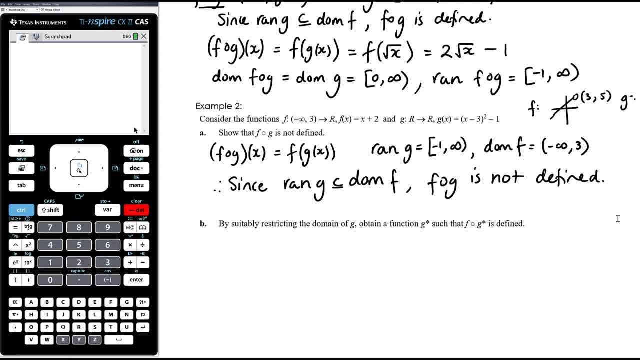 about it being a subset or not being a subset. so make sure you're using sort of appropriate mathematical language and notation when you're writing things down and you're answering questions. but you know we can have a more flexible understanding of that in terms of the way we 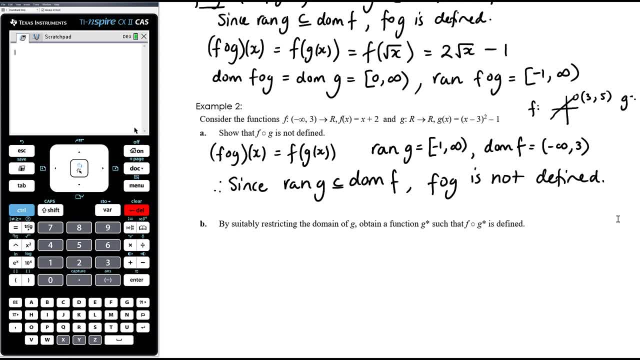 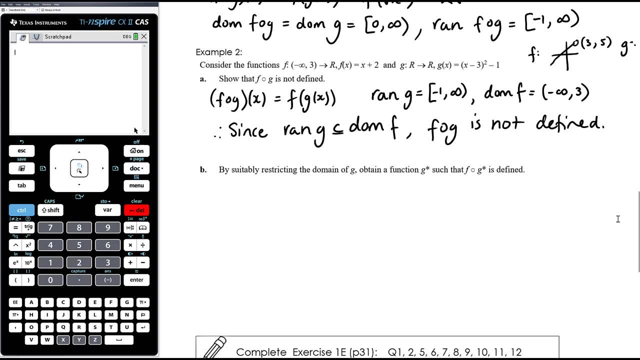 talk about it verbally to help you understand what's happening. so the problem at the moment is that the range of g includes numbers in it that are not in the domain of f. okay, so at the moment, g of x, we know, is um, a parabola, with its turning point at three negative one. okay, uh, i'm just 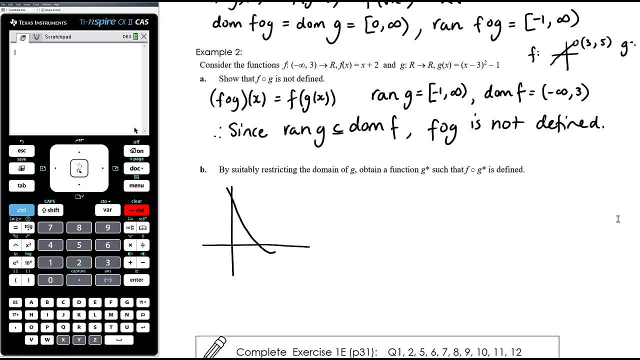 thinking about: yeah, okay, and at the moment we need, we need for the composition to exist, we need the range of g to be able to fit into negative three to negative, infinity to three. now we're not going to be changing where the turning point is. we're going to be changing where the turning point is. 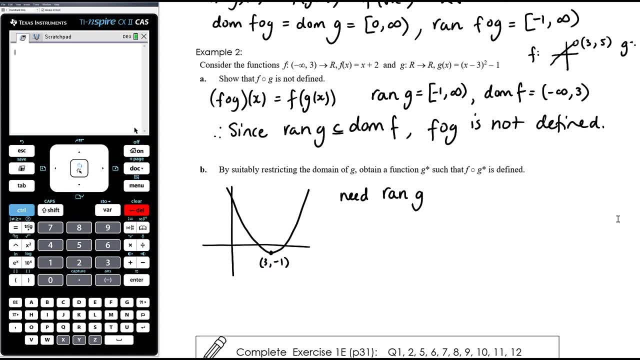 we're not translating the graph, we just want to restrict its domain. so the domain currently goes from: sorry, the range currently goes from negative one up to infinity, and the problem is is that we need it to stop at three so that it will be a subset of the domain of f. okay, so sorry, i'm. 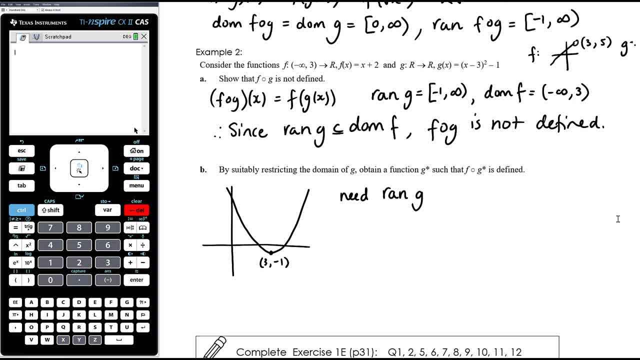 raising that. let's try again. so we need the range of g to be equal to. we can't change the negative one. sorry, it's going to go from negative one, but we want it to stop at three and it can't include three because three isn't included in the domain of f. so we need to stop. 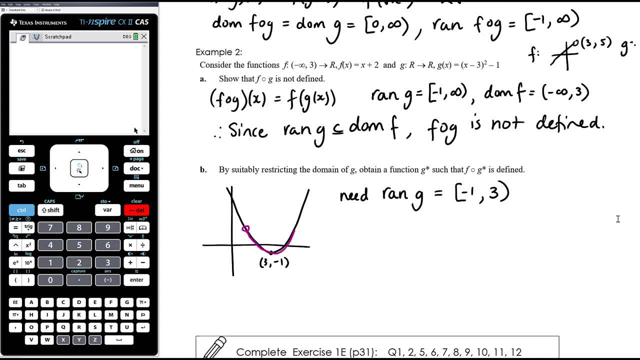 at three, wherever three is, we need this to be the function g. okay, so this is y equals g, g of x. sorry, all right, so we need. we need that to be y equals three. okay, so that um, its range is now just negative, one to three, not inclusive, and then if its range is that, that will be a subset of 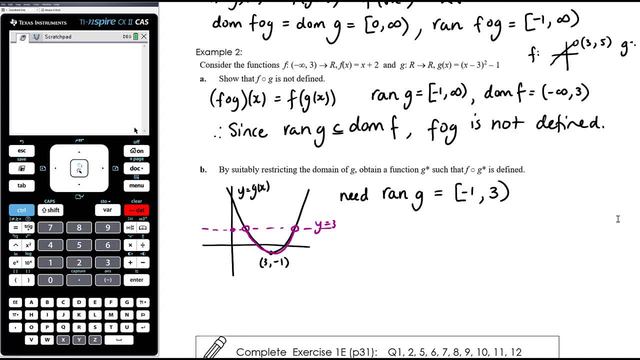 negative infinity to three, not inclusive, and therefore the composition will exist. so sorry, we need the range of g star to be that which is our modified version of g. okay, so to work out, but we can't restrict a function by restricting its range. that's not how functions work. function is about domain, and rule x values what you do to them. so we need to. 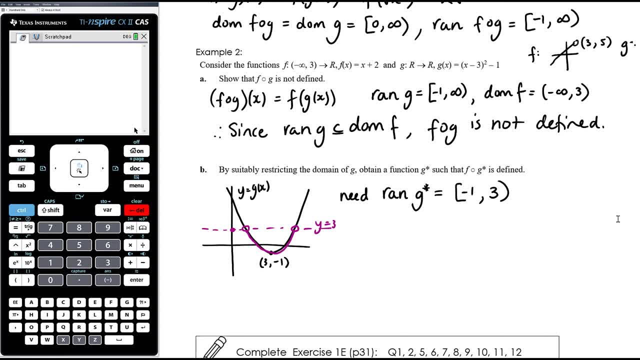 work out, okay. well, what does this mean for the x values? so that we only get a range that goes from um negative one up to three, which means we want to restrict the domain of our function to just be between these two x values here. okay, so we need to work out what those are. so we need